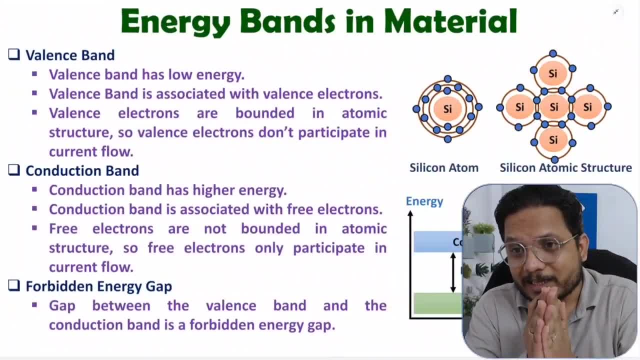 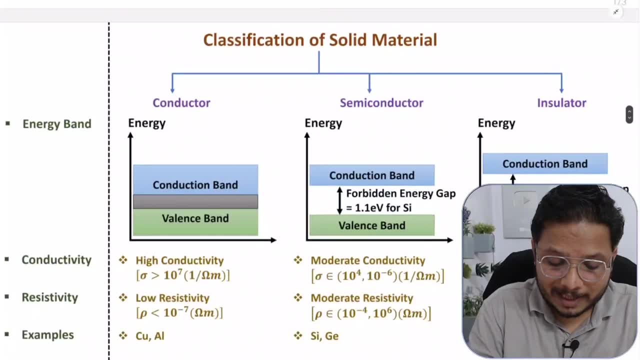 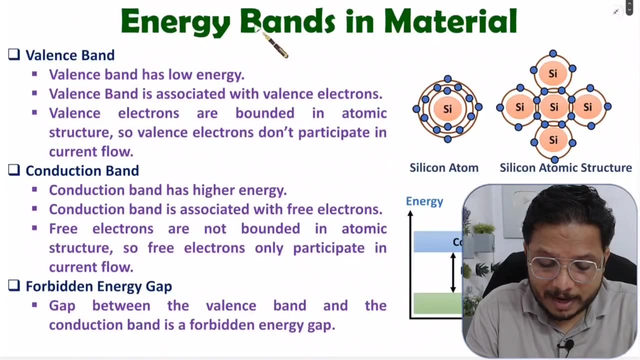 Hello friends, welcome to engineering funda family. In this video I'm going to explain you energy bands as well as I'll explain you how classification of solid material is there with respect to energy bands. So first of all, I'll explain you energy bands in material. 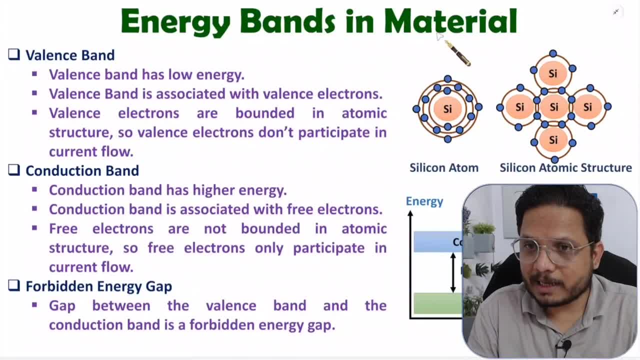 Basically, there are two categories of band available with material in terms of energy bands: valence band and conduction band, See valence band. valence band that is associated with valence electrons and conduction band that is associated with free electrons. So 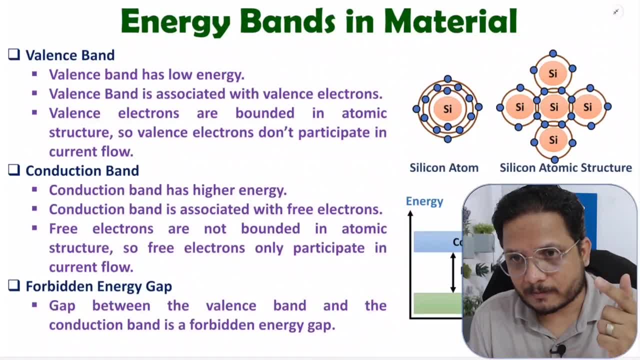 first of all you need to understand what is the meaning of valence electrons, See valence electrons are the electrons which are bounded in its atomic structure, Like as if you talk about one silicon atom over here, then you can observe in the silicon atom with first. 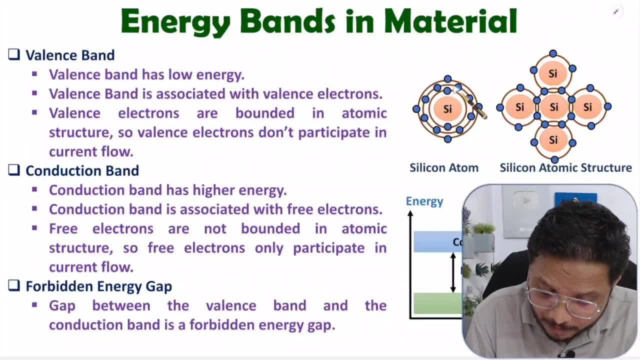 orbit, We are having two electrons. with second orbit We are having eight electrons. with outermost orbit We are having four electrons. So these are the electrons which are bounded in its atomic structure. If you observe atomic structure of silicon, then there are covalent bonds. 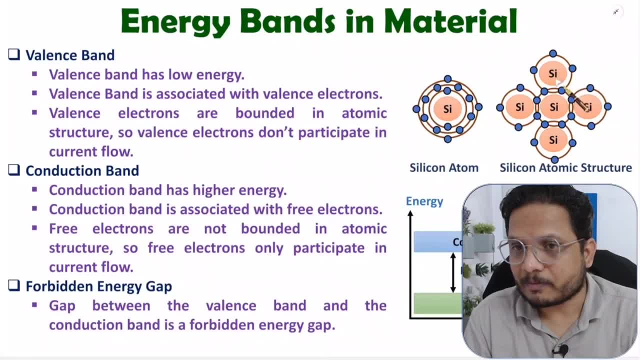 by which these electrons are connected with each other. So the electrons which are connected in its atomic structure, those are valence electrons, And the electrons Which are not connected in its atomic structure, those are free electrons. So here we see valence. 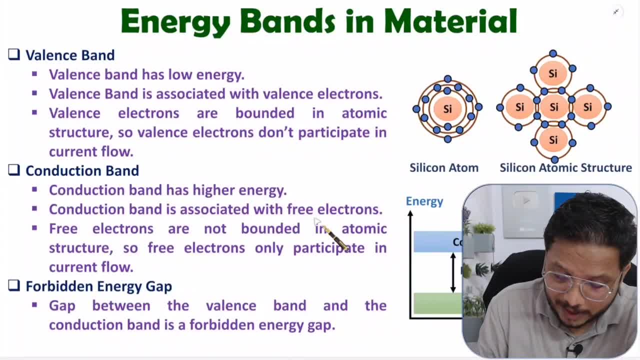 electrons that will define a valence band and free electrons that will define conduction band. So first of all you should be having idea about what is valence electrons? See valence electrons are connected in its atomic structure And three electrons are not connected in its atomic structure. So two electrons participate. 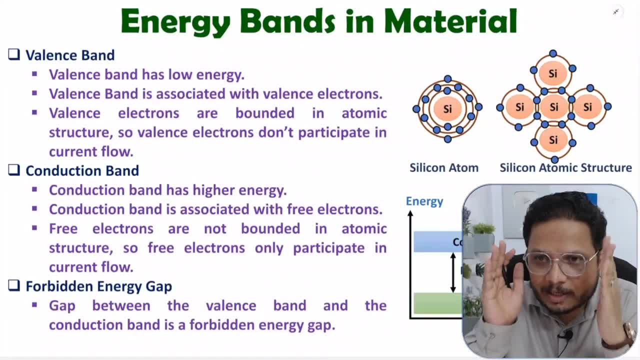 in iling. So whenever you apply potential difference in between two terminal of material, then there is a possibility of flow of current and that flow of current is possible due to free electrons only always remember this valence: electrons does not participate in flow of current right. 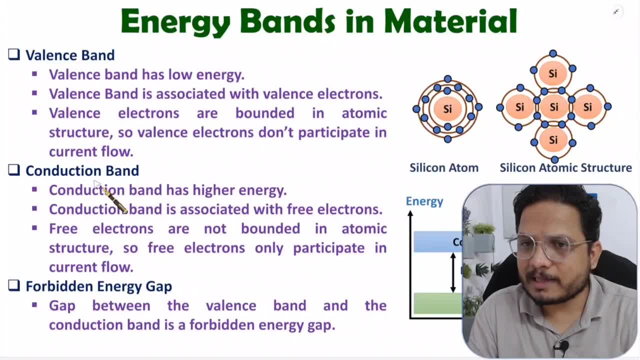 So let me explain you how valence band and conduction band is there now. valence band energy will be always low. why it will be always lower? the reason is: valence band is associated with valence electrons and valence electrons are bounded in a bond of atomic structure. 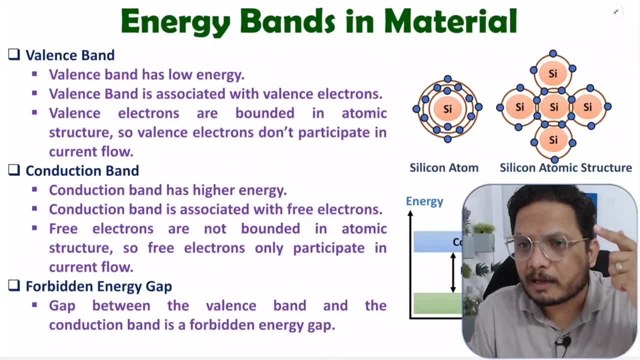 as those electrons are bounded, those electrons are having lower energy and because of that, valence band will be having low energy. valence electrons are bounded in atomic structure, so valence electrons does not participate in flow of current. Well, when you talk about valence band, 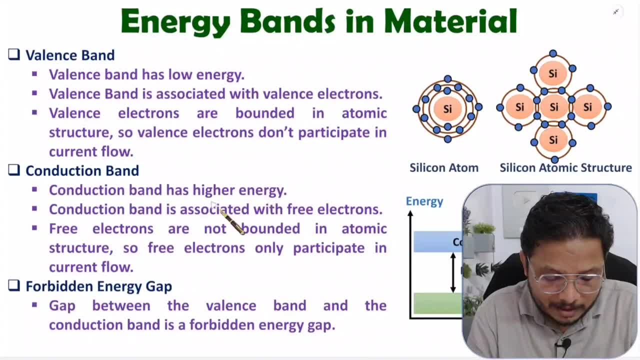 When you talk about conduction band, conduction band is having higher energy. the reason is conduction band is associated with free electrons and free electrons are not bounded in atomic structure, so free electrons only participate in flow of current. So first of all you should know in structure there are two types of electrons, right? the? 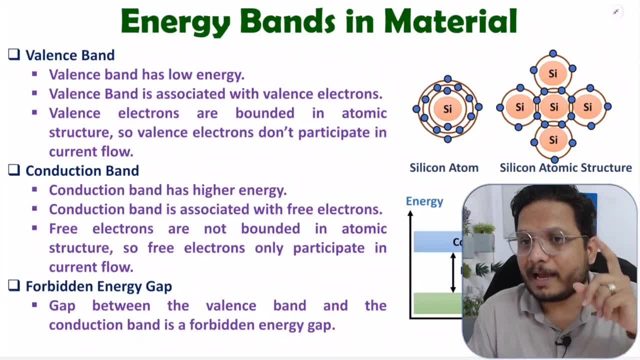 electrons which are bounded in the structure. those are valence electrons. energy associated with valence electrons is valence band. that energy will be low. Free electrons are not bounded in the structure. energy associated with free electrons will be there in conduction band and that will be having higher energy. right now, when you 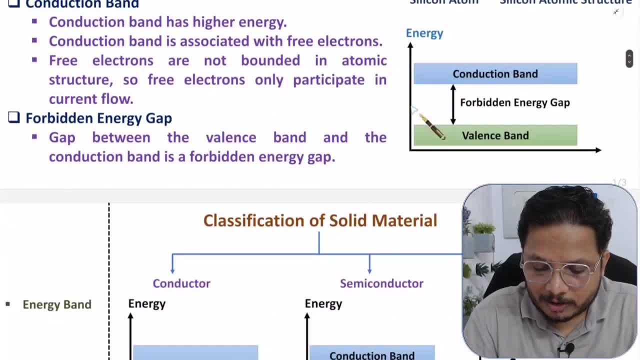 talk about energy, then here you see, I have drawn energy band diagram. so here conduction band energy that is high. I have told you why the reason is: conduction band energy that is associated with free electrons. valence band energy that will be low. Why the reason is: valence band energy that is associated with the electrons, which are 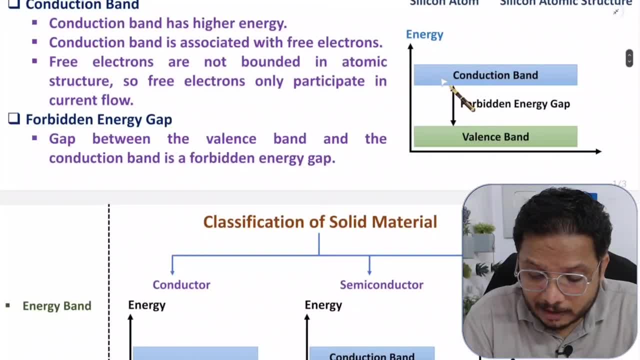 bounded in the structure. gap in between conduction band and valence band is referred as forbidden energy gap. now what is the meaning of forbidden energy? see, in valence band there will be electrons. let me draw some electrons over here. see, in valence band there are few electrons right now. see, 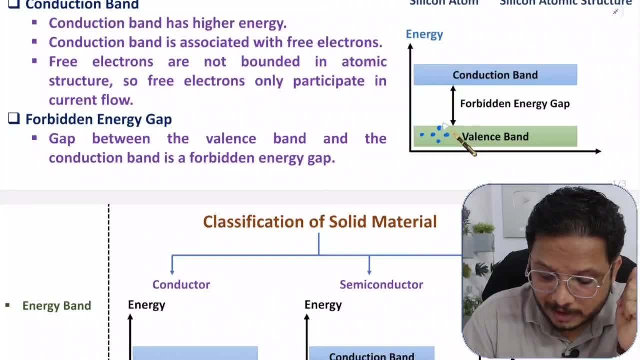 to have flow of current. if i want to move these electrons in conduction band, then how much energy that i need to give it to this electron? that is what forbidden energy gap. see, if you have a material in which there is no free, there is no free electron, then is it possible that there can. 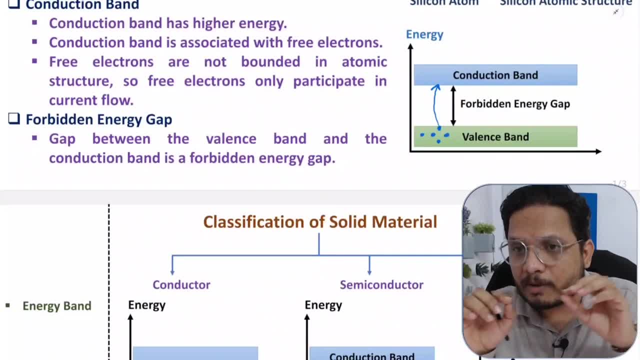 be flow of current. if there is no free electron then there cannot be flow of current. but if you increase potential difference in between material, then these electrons will gain energy and as if these electrons jumps into the conduction band, means now those electrons are getting free, then those electrons which are there in conduction band, they can only participate in flow of current. 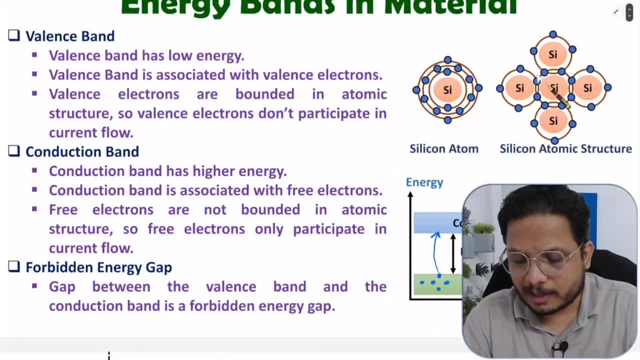 so here you see this atomic structure that is having electrons which are valence electrons, so these electrons cannot participate in flow of current, but as if i give energy to electrons, like as if i give energy to this electron and as if i make it free, as if i make it free. 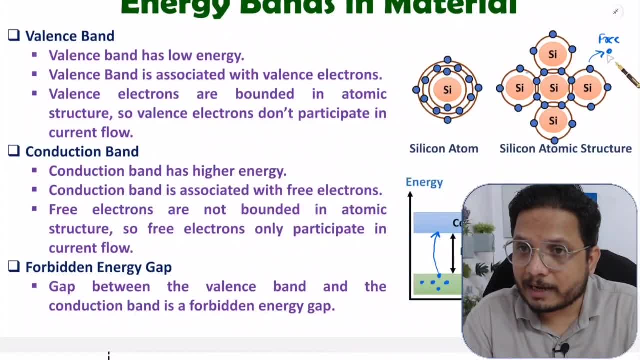 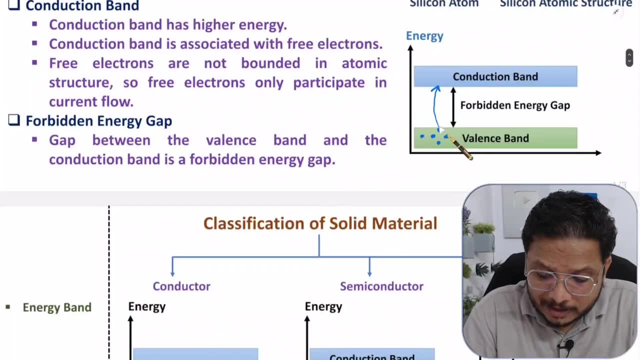 right, then this electron will go in conduction band and that electron can participate in flow of current. so to give, so to give energy to electron here we need to give some electric field, or we can give some potential difference, or you can provide heat as well there. 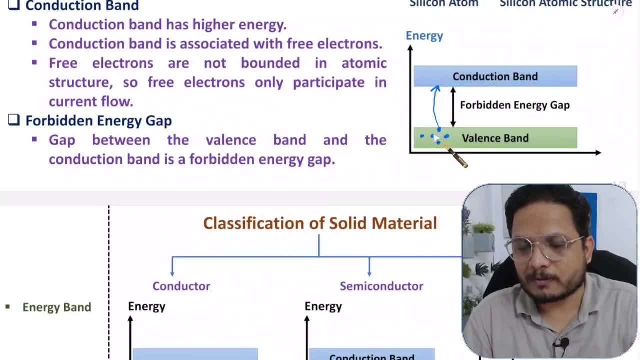 are multiple ways by which we can give energy to electrons. either you give heat to material or you can provide potential difference in between material, as well as you can provide high electric field to material, by which you can transfer this valence electron into conduction band, and you can 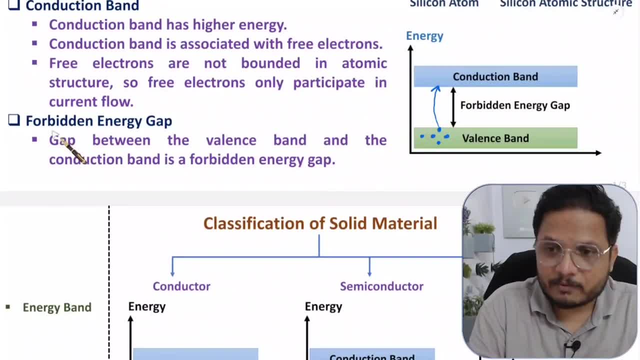 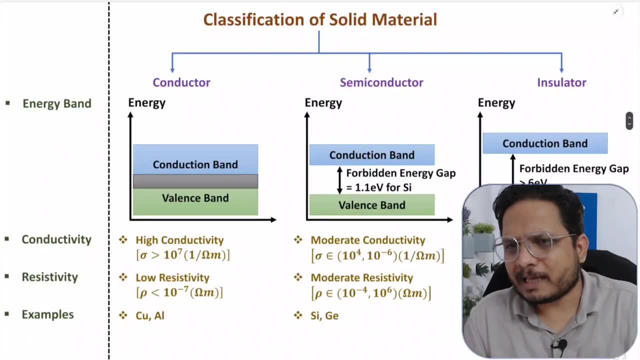 make it free and this gap is referred as forbidden energy gap. now let me explain you. how classification of solid material is there? probably, i think you might be having idea about what is. what is conductor, semiconductor and insulator? right, still, let me tell you see, in conductor we are having 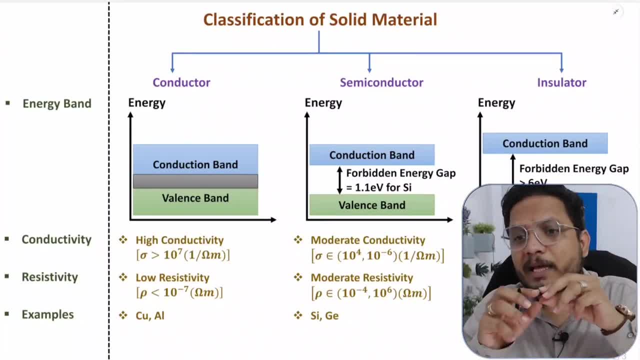 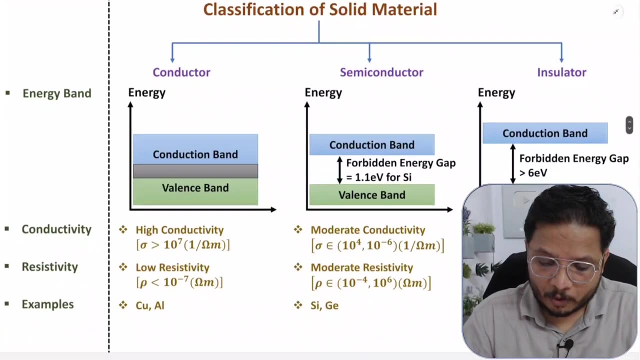 higher conductivity means easily we can flow current inside conductor. in semiconductor you will have to give more energy for a flow of current, while in insulator it is bit difficult to flow current. why? the reason is forbidden energy gap. that is very high if you observe energy band diagram over here. 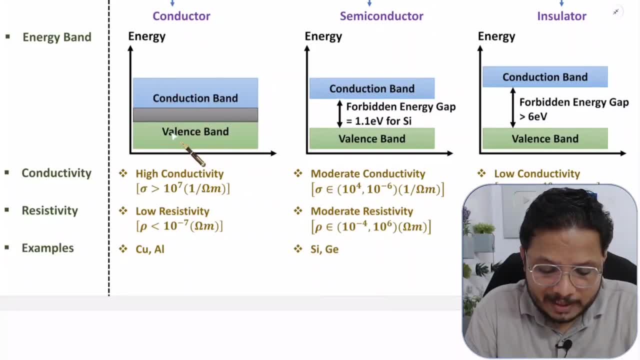 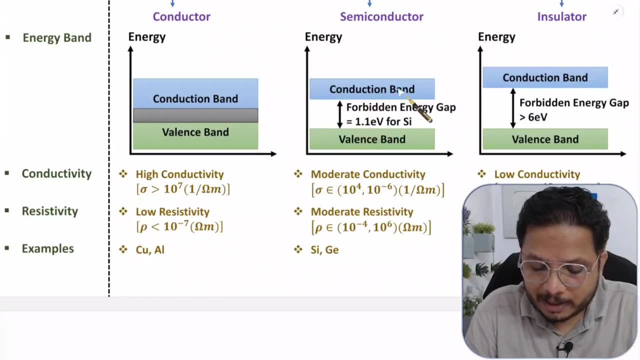 you see, with conductor conduction band and valence band that is overlapped over each other. as it is overlapped over each other easily, flow of current will happen by applying potential difference. as if you talk about semiconductor, then forbidden energy gap in between conduction band and valence band. that is bit low. for silicon it is around 1.1 electron volt. 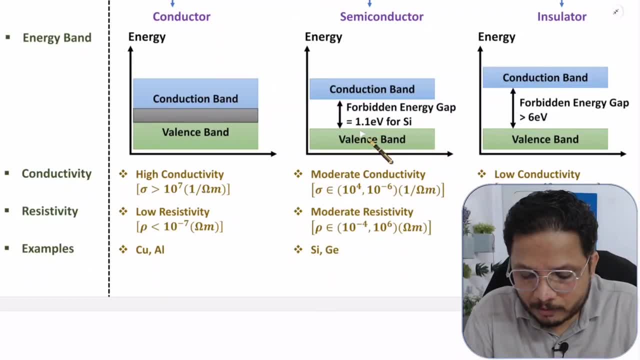 right. so with silicon material if you give 1.1 electron volt energy to one electron, then that electron will jump from valence band to conduction band and those electrons can participate into flow of current. but if you talk about insulator, so in that if you observe here forbidden energy gap, that 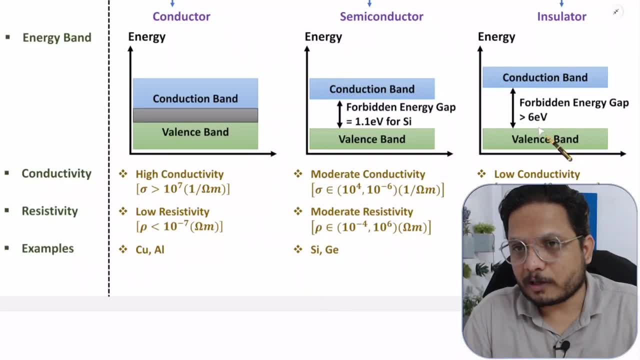 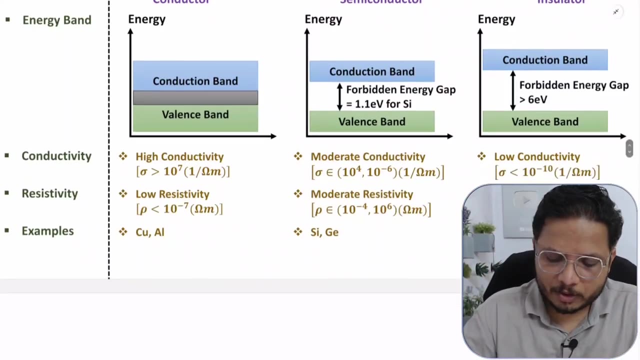 is very high. it is greater than 6 electron volt. so as forbidden energy gap is very high in insulator, there will be no flow of current, even if you apply some potential difference in between two terminal of material. here there are few parameters that you need to understand. 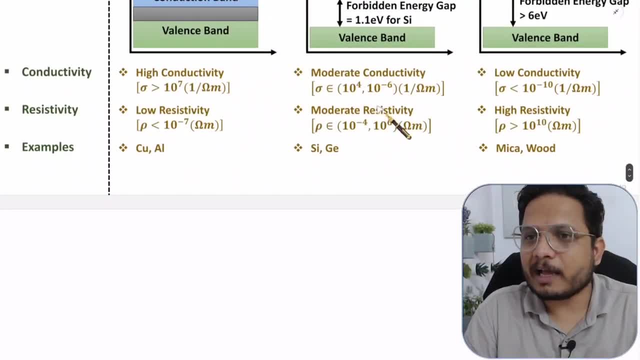 and i have seen- see this- parameters that frequently comes in competitive examination. so you should remember those parameters right, like: how conductivity is there? so with conductive material, high conductivity will be there. with in with semiconductor, moderate conductivity will be there, and with insulator, low conductivity will be there, see with conductor conductivity that is. 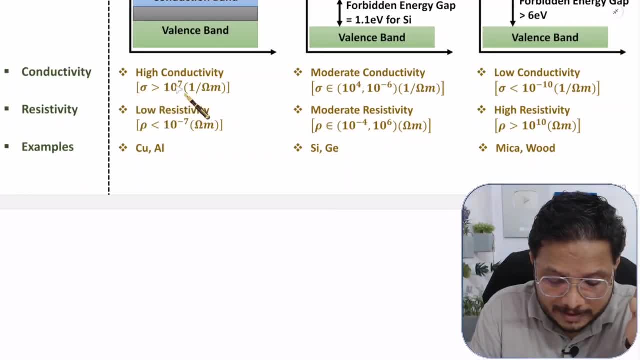 represented by sigma and that will be greater than 10 to the power 7 per ohm meter. see this sigma that is having unit which is per ohm meter. remember, this sigma is having unit that is per ohm meter and will be greater than 10 to the power 7.. if you talk about semiconductor material, then this sigma 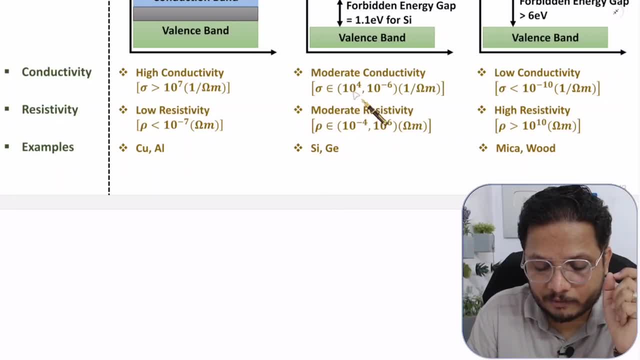 conductivity that will be there somewhere in between 10 to the power 4 to 10 to the power minus 6 right, and for insulator that conductivity will be very low. that will be there in terms of 10 to the power minus 10 per ohm meter. so based on conductivity also you can classify those materials. 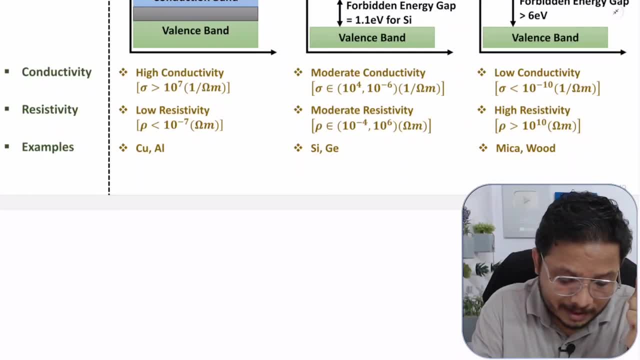 based on resistivity. also we can classify the material. now, what is the relation in between conductivity and resistivity? see, conductivity is inversely proportional to resistivity. so sigma that is inversely proportional to rho means sigma is proportional to 1 by rho. so you can observe here: unit is ohm meter with conductivity unit is per. 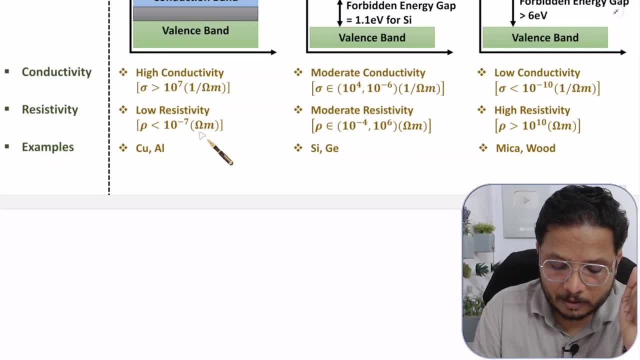 ohm meter with resistivity unit is ohm meter right. so rho that will be lower than 10 to the power minus 7 for conductor. so it will be having lower resistivity. moderate resistivity will be there with semiconductor material right and high resistivity that will be there with insulating. 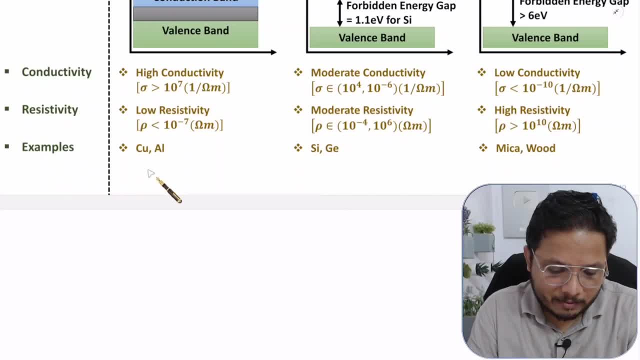 materials. some examples that i have written over here. like with conductor, we can have copper, aluminium. those are not ideal conductor, but you can say those are conductors that is, having good conductivity for semiconductor- silicon and germanium that people are widely using nowadays. so if you talk about semiconductor chips, then that is made up of silicon material only and as if you 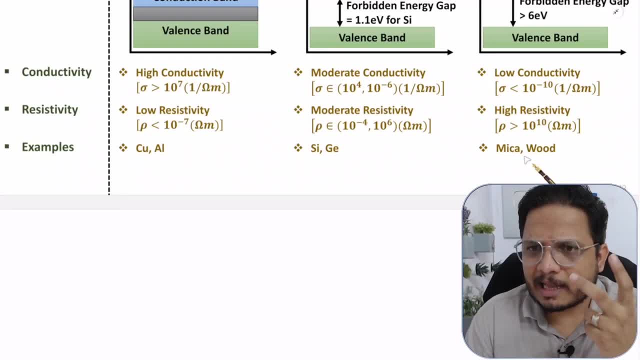 talk about insulating material, then mica wood, right. so those are the real life examples of insulating material. so here there are few basic points that you need to note down. see, first of all, what is the meaning of valence band and conduction band and what is forbidden. 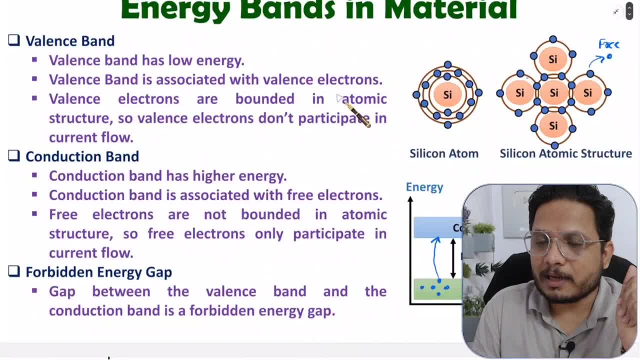 energy gap. valence band that is associated with valence electrons, and valence electrons are there as part of the atomic structure as per some bonds right, and conduction band that is associated with pre-electrons. pre-electrons are free. those are not connected in atomic structure, so those 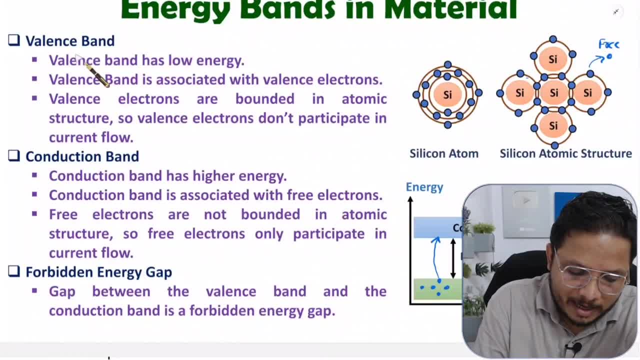 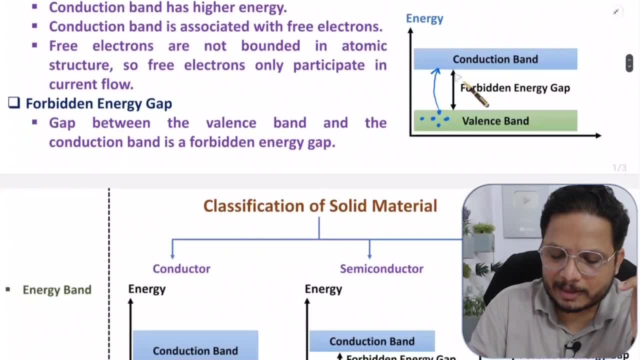 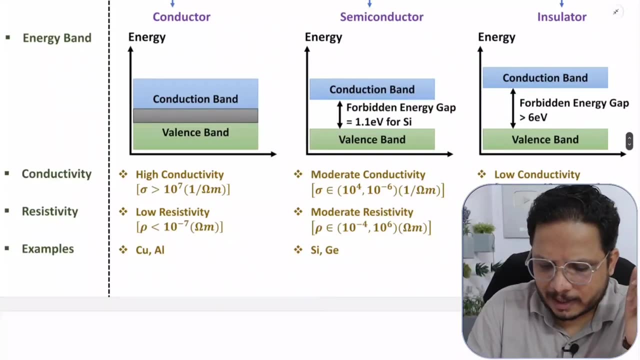 electrons which are free, they can participate in flow of current valence band will be always having lower energy. conduction band will be always having higher energy right. and here one example i have given over here diagram you should note down, see, with insulator, forbidden energy gap, which is a gap in between.